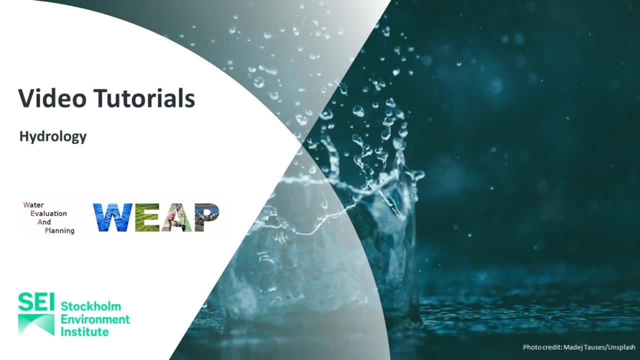 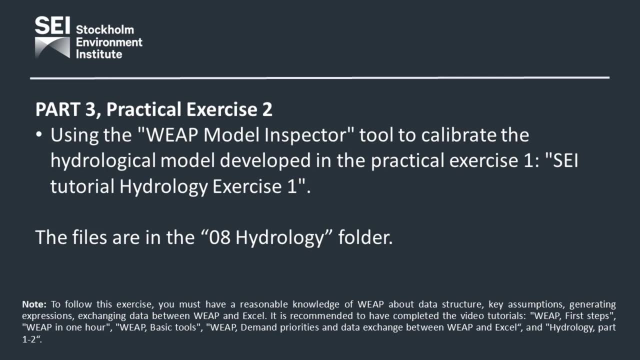 Hello, This session is the second exercise of the hydrology video tutorial. We developed a hydrological model using the soil moisture method. in the first exercise We added the rivers, catchments, runoff, infiltration links and stream flow gauges. We characterized the catchments by entering area, climate and land cover classes. 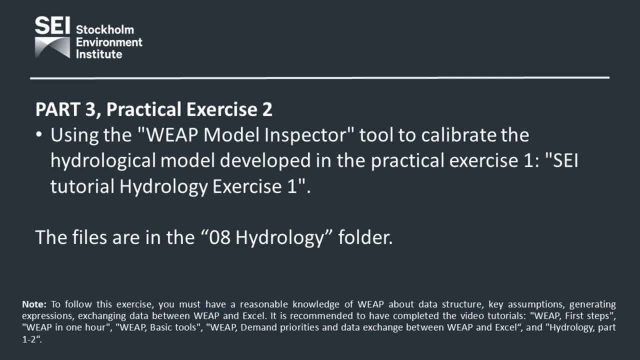 We created key assumptions to manage the hydrological parameters and assigned them to each catchment. In this exercise, we will see how to use the WIP model inspector tool to calibrate the hydrological model developed in the exercise. 1. The tool has embedded macros to 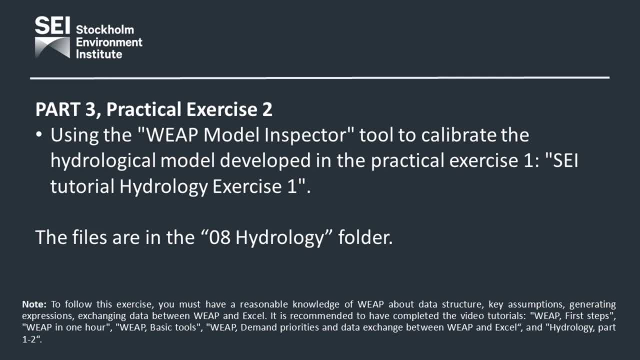 exchange information with WIP, It is recommended to have followed all the sessions of the hydrology video tutorial. If you are interested in learning more about the hydrology video tutorial, please subscribe to the channel. You will need to download the 08 Hydrology folder to follow this. 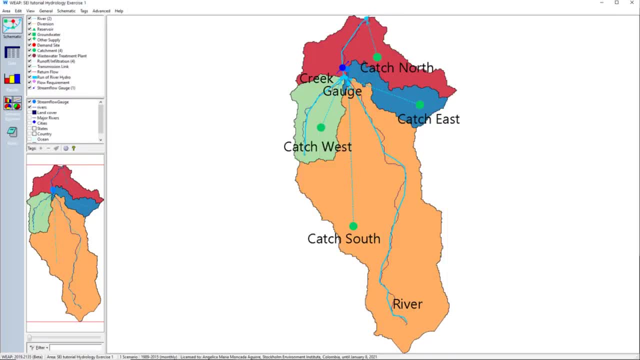 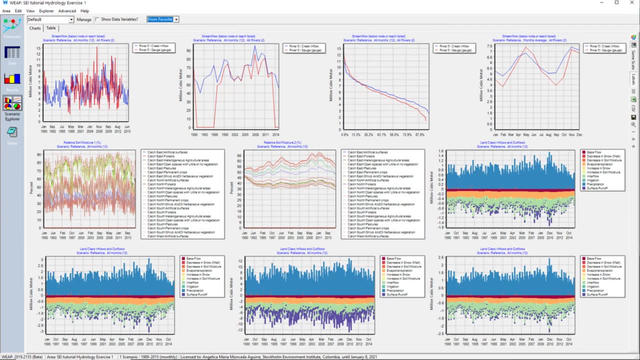 exercise. In the exercise 1, we developed this model. We were exploring the results by comparing the observed versus simulated stream flow. Once we have completed the hydrological model, before using it to build scenarios or assess the available water resources, we must calibrate and validate the model. We will use the WIP model inspector tool. 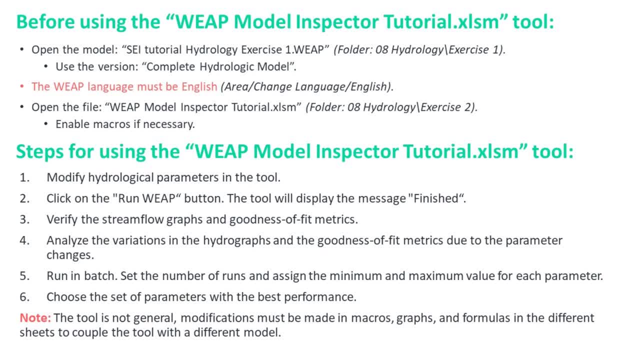 Before using the tool, we need to open the complete hydrologic model version of the SEI tutorial hydrology exercise 1 model. If you have WIP in other languages rather than English, you must change it to English. The WIP language must be in English. 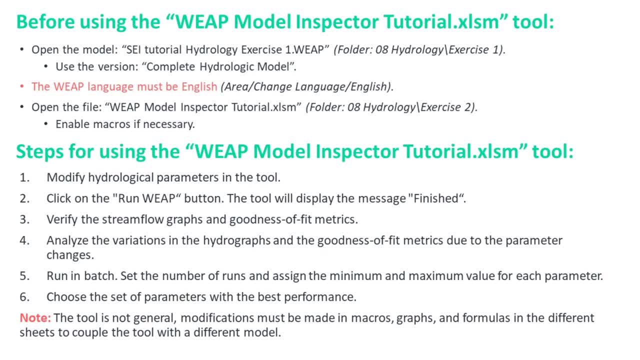 because the macro code uses the name in English of the WIP elements, variables and results, We need to enable the macros in the WIP model inspector tutorial file. We will follow these five steps to use the tool. First, we need to modify the hydrological 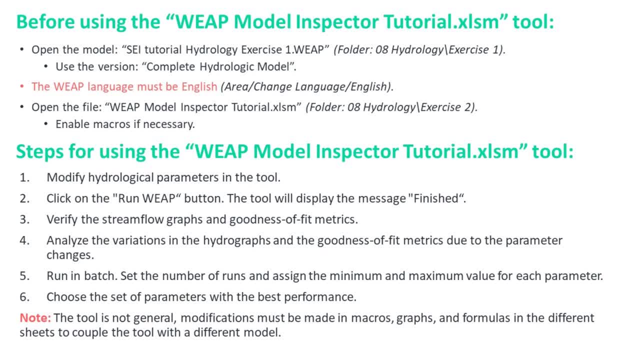 parameters in the tool, not in WIP. Second, execute the macros by clicking on the Run WIP button. The run time depends on your computing capacity. Third, verify the streamflow graphs and goodness of fit metrics. The graphs should be used to: 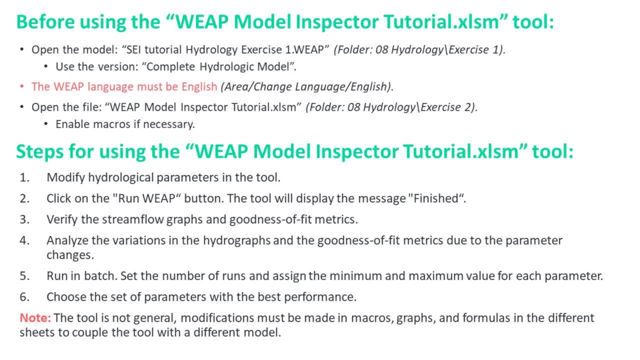 understand the hydrological response to changes in the parameters, For example, if the peak flows increase or decrease. if the base flow increases, if the response is slower or faster, The tool can run in batch. The end set of parameters are constructed by. 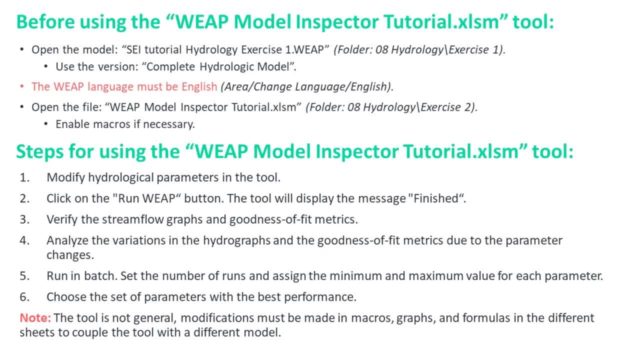 generating random numbers between a minimum and maximum value for each parameter. Fifth, choose the best set of parameters based on goodness of fit metrics and water balance results. Remember that the tool is not general. Modifications must be made in macros, graphs and formulas to couple the tool with a different model. The tool was already modified. 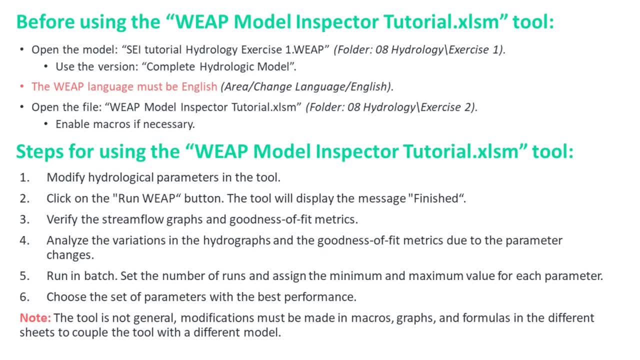 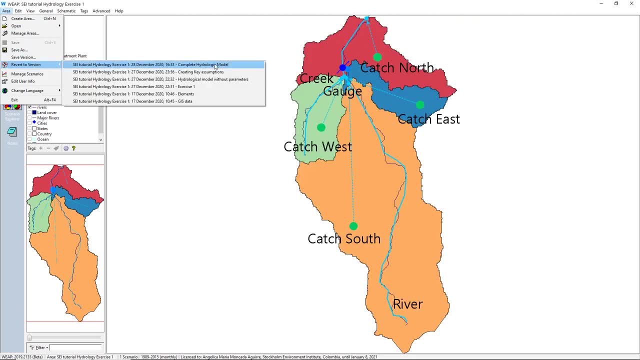 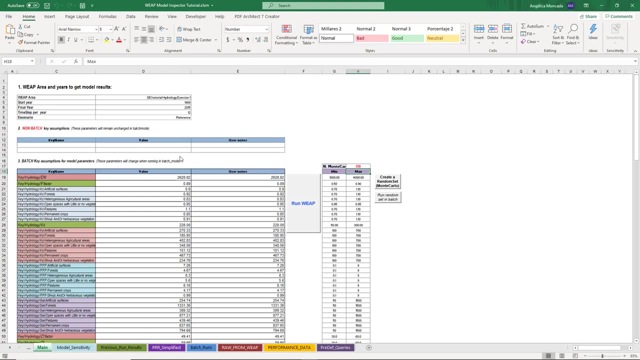 to work on the SEI tutorial: hydrology exercise 1 model In WIP. go to area, reverse to version and open the complete hydrologic model Version. We have the model opened and the tool ready to use. The instructions to use the tool. 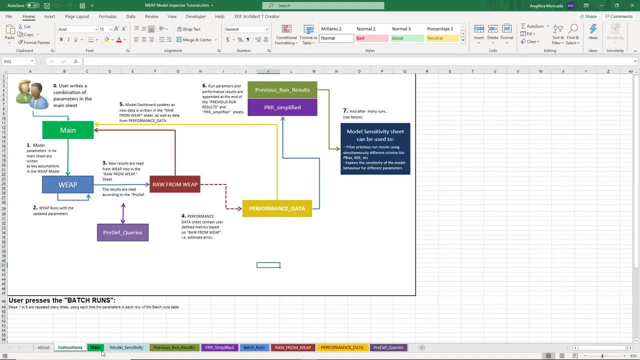 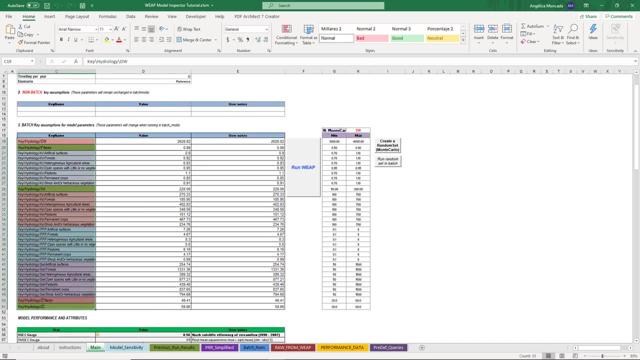 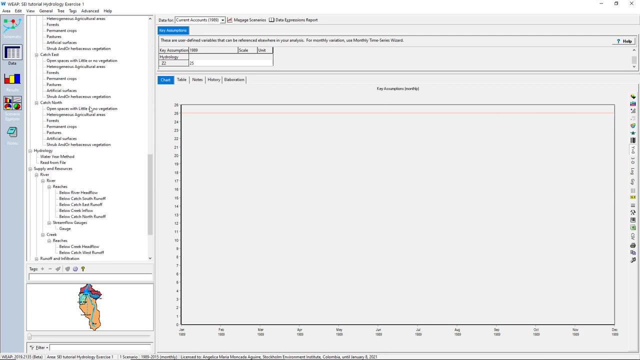 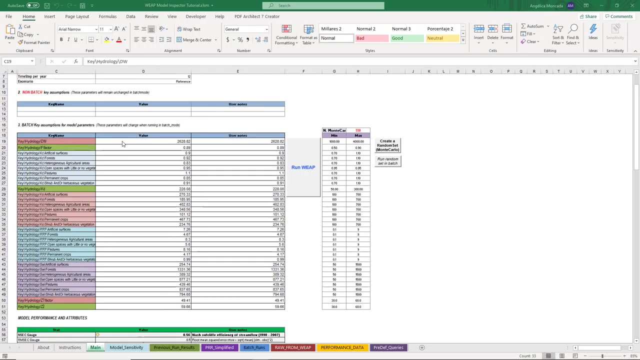 are in this sheet. In the main sheet you will find the list of the hydrological parameters created in the SEI tutorial hydrology exercise 1 model. The hydrological parameters are controlled by key assumptions. You can change these key assumption values from this tool via macros. For example, change deep conductivity from 228 to 150. 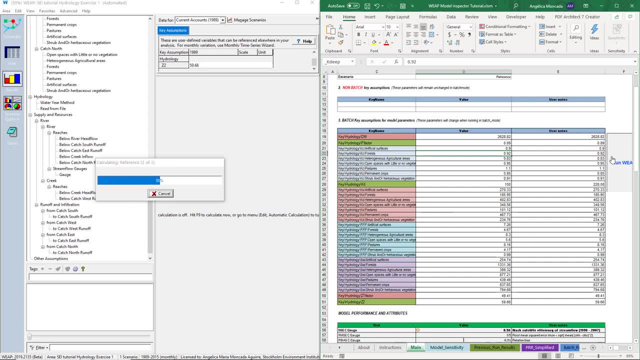 Click on Run WIP, The tool starts assigning these values to the key assumptions in WIP. Then the model will be run and the tool will import the results. When the macro finishes, a pop-up will appear When the macro finishes. a pop-up will appear When the macro finishes. 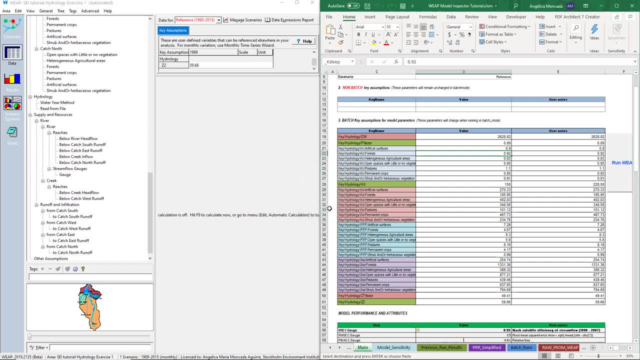 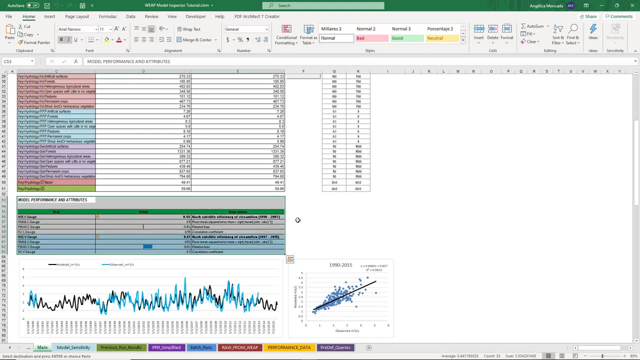 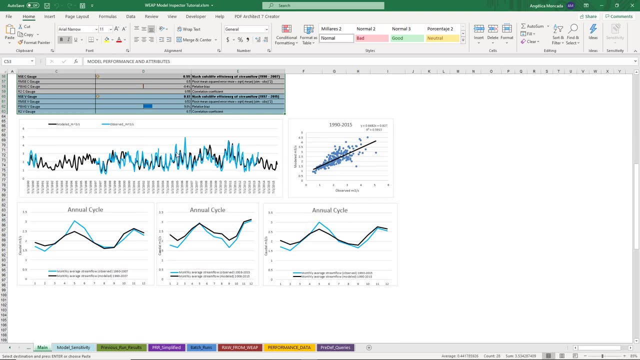 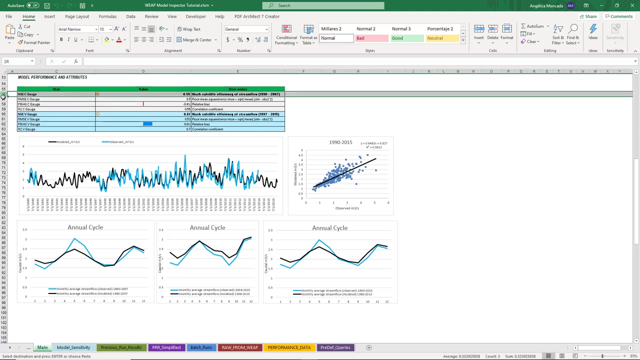 a pop-up window will appear. You can access the model performance for the last run in this section. The tool displays these graphs comparing the observed and the simulated streamflow and the goodness of fit. metrics for the calibration and validation period: The Nash index, the root mean, squared error, the bias and the correlation coefficient. 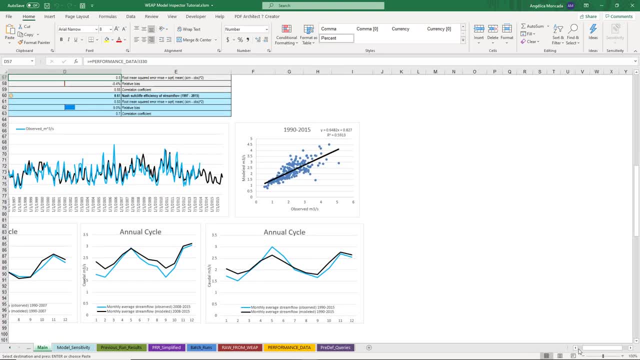 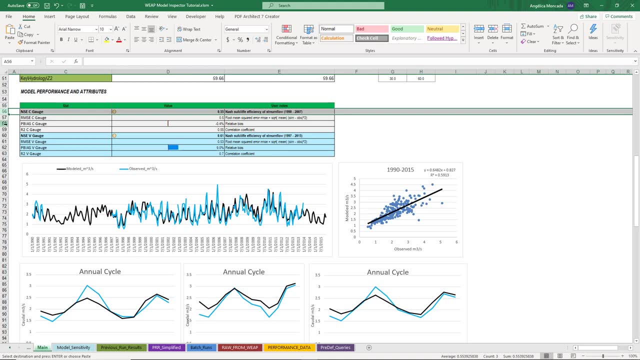 are shown. You can modify the tool and include other goodness of fit metrics. Regarding the Nash index and correlation coefficient, the closer to 1, the better the model performance. Meanwhile, the bias and the root mean squared error the closer to 0,. 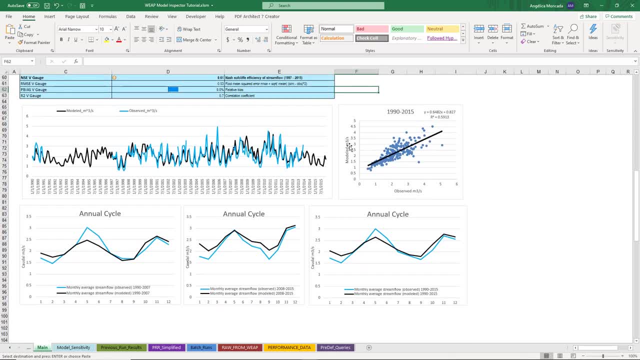 the better the model performance. We can see on these graphs how well the model performance has improved over the years. We can also see how well the model performance has improved over the years. The time series, the annual cycles and the scattered plot are shown. 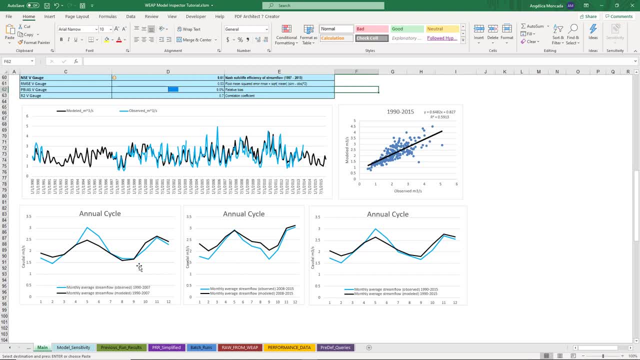 In this case we use the split sample test. We split the modeling period into two: 1990 to 2007, and 2008 to 2015.. Each time the tool runs the least of the parameters and the goodness of fit metrics. results are saved in the previous 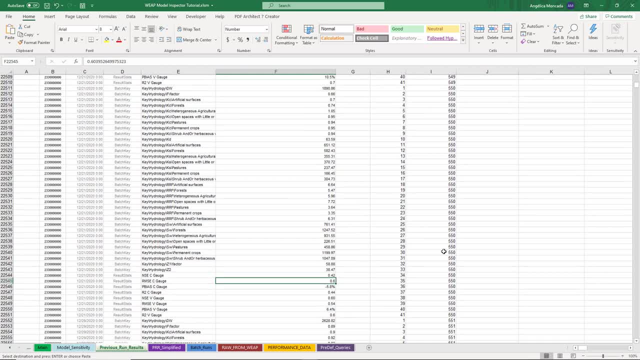 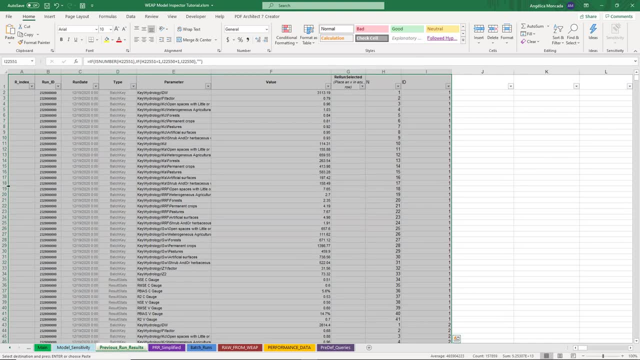 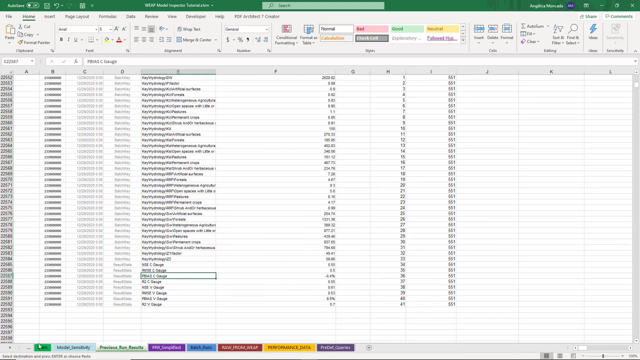 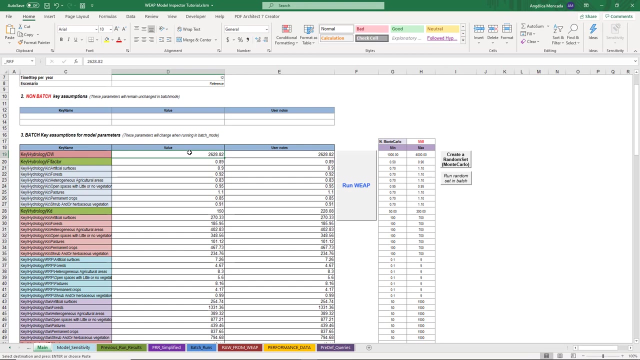 run results sheet. The tool was used previously 550 times. We just run it one more time and now we see 551 records. For example, change the work capacity from 2,620 to 3,598 to 3,500 and run the tool again. Click on the Run Whip button. We will have 552 runs. 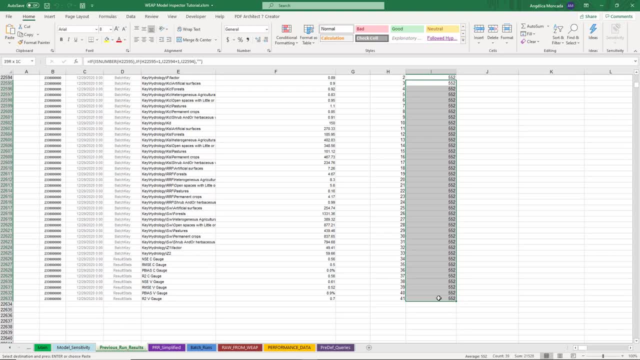 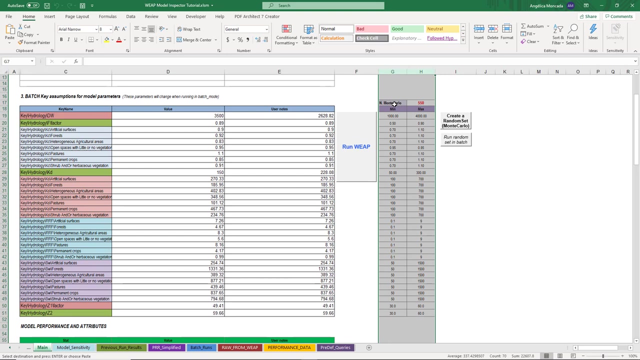 The tool is useful to evaluate the hydrological response due to parameter changes. We can run the tool in batch. We will test five sets of parameters using this feature. Go to the main sheet. We will use the G and H columns First. in the H17 cell we need to set: 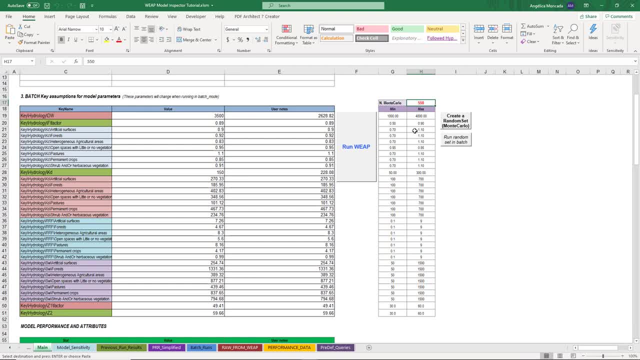 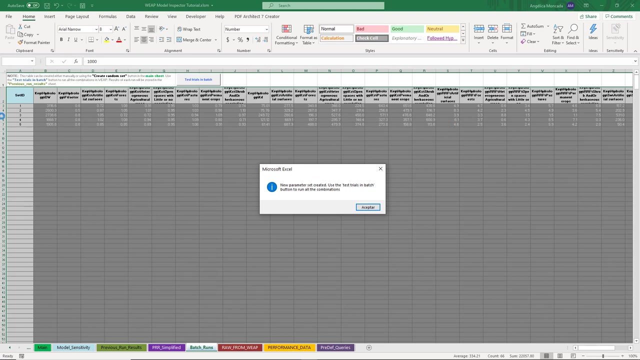 the number of runs, In this case five. Next, we set the minimum and maximum values to define the interval at which random numbers will be generated for each parameter in the list, Click on the Create a random number Set button. The tool generates random values for each parameter in the batch runs sheet. 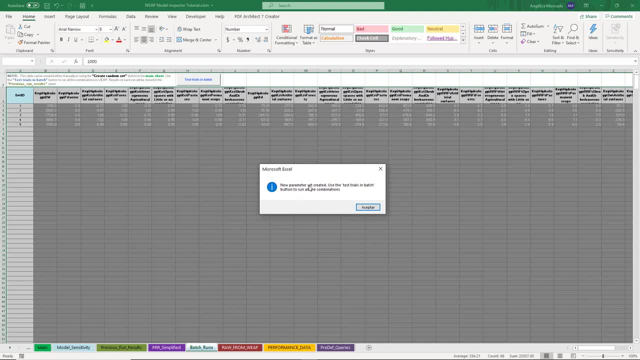 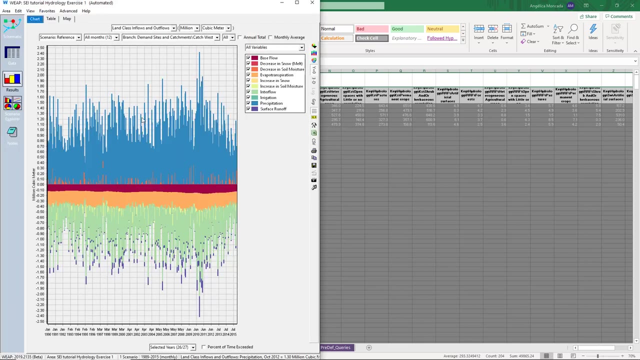 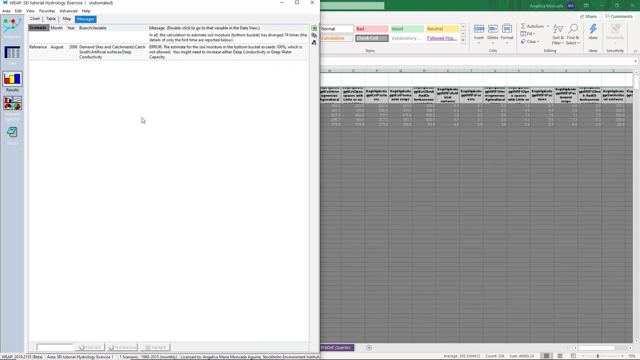 It will appear in a pop-up window. New parameter set created. Use the Test trials in batch button to run all the combinations Accept. Click on the Test trials in batch button. The run time depends on the number of runs, the complexity of the model and the computer capacity. 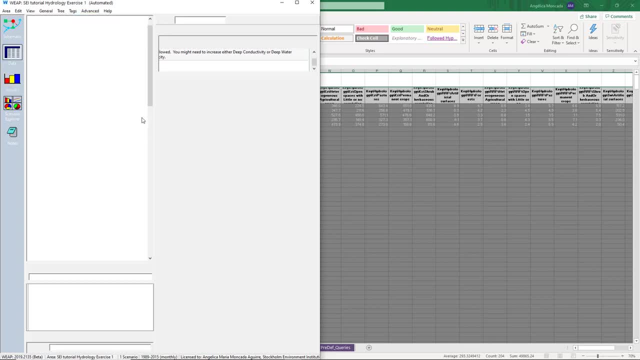 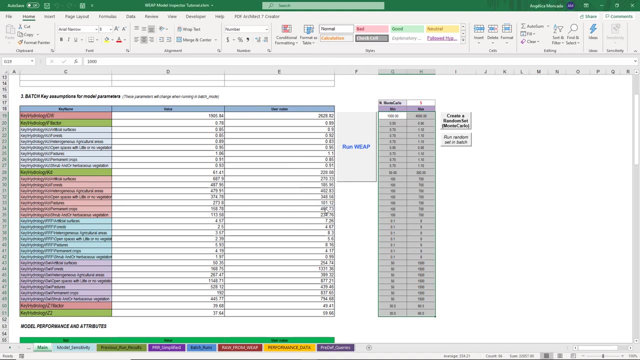 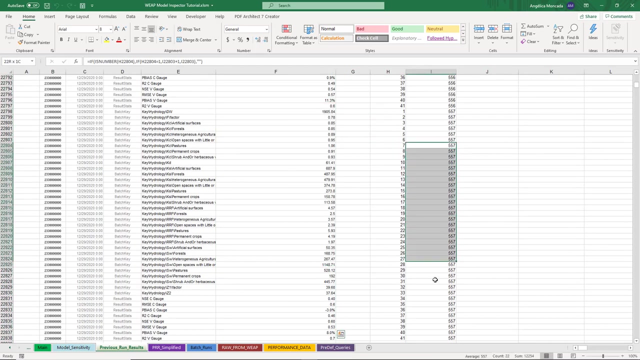 Each row represents a set of parameters. The tool starts assigning those values to the key assumptions in batch. When it finishes we can check in the previous run results that there are five more records. We have the results from 557 runs- The advantage of having the goodness of fit metrics for several sets of parameters. 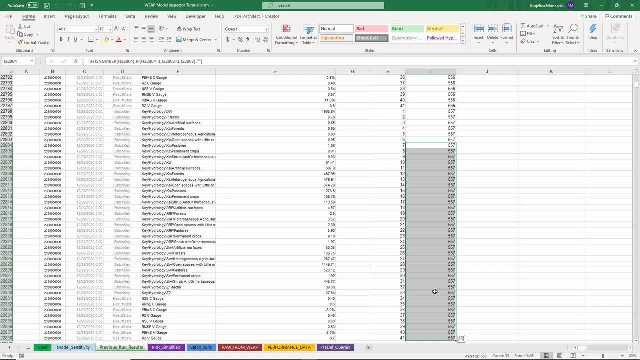 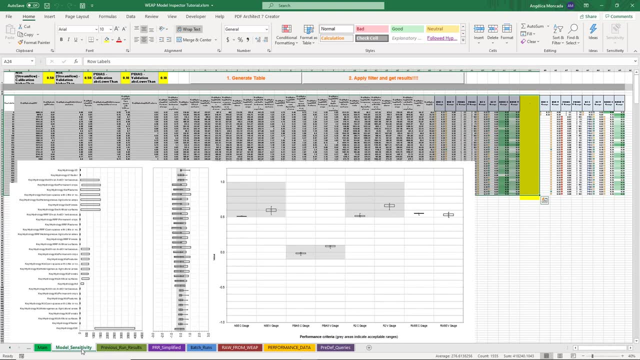 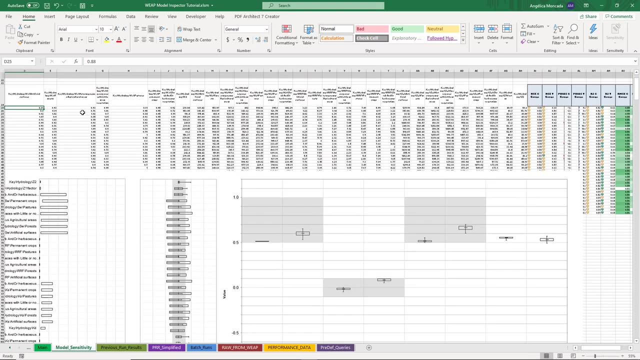 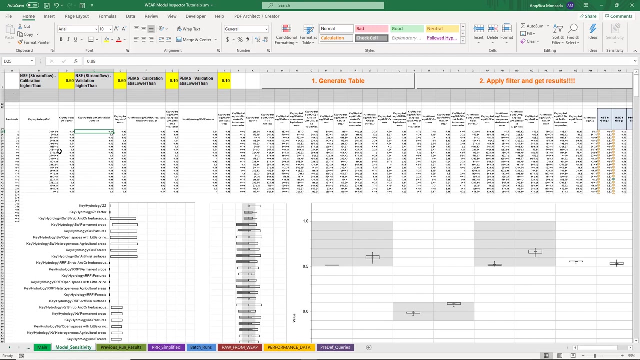 is to evaluate which sets meet the performance criteria. Go to the model sensitivity sheet. We use this sheet to organize the previous results in a table and apply the performance criteria to the results so that we filter the sets of parameters. The filter results are based on the table. After running the model, you must update the table first. 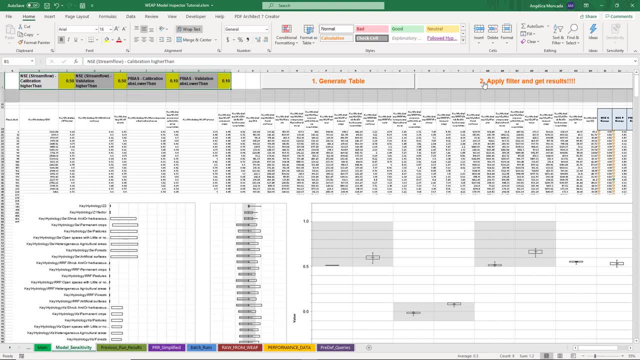 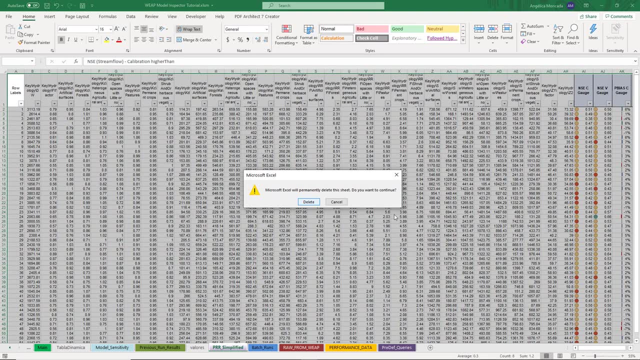 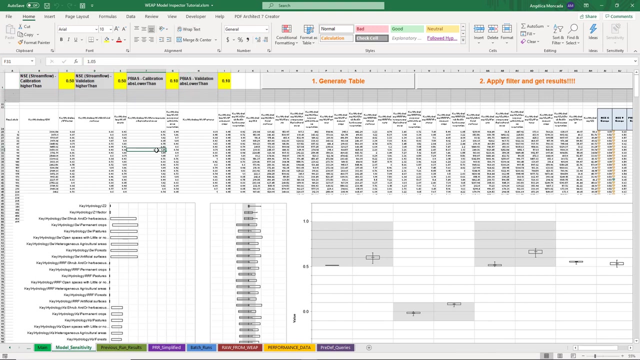 Then you can apply the filters. Click on the Want generate table button. The tool may display a warning indicating that a sheet will be deleted. This is related to the code and is normal. Click on the Delete option. We can now apply the filters. We are going to get the sets of parameters. 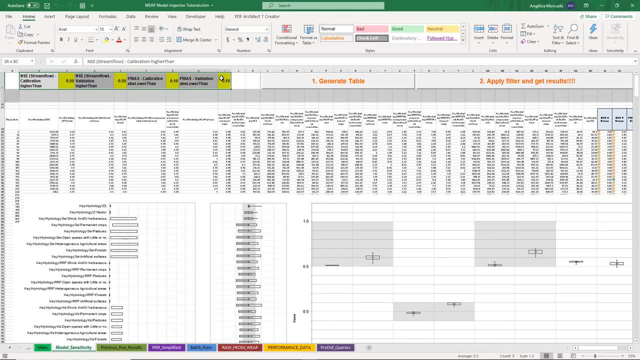 that meet these performance criteria, The Nash index in calibration and validation will be greater than 0.5 and the absolute value of the bias index will be lower than 10%. Click on the To apply filters and get results button. As we see, some sets of parameters meet this condition. 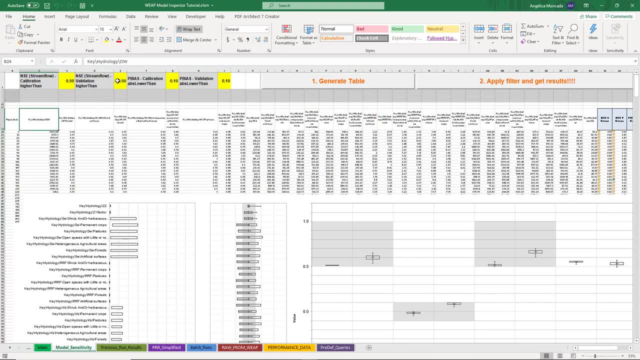 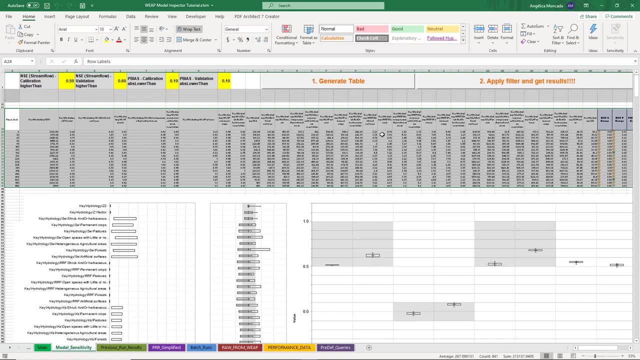 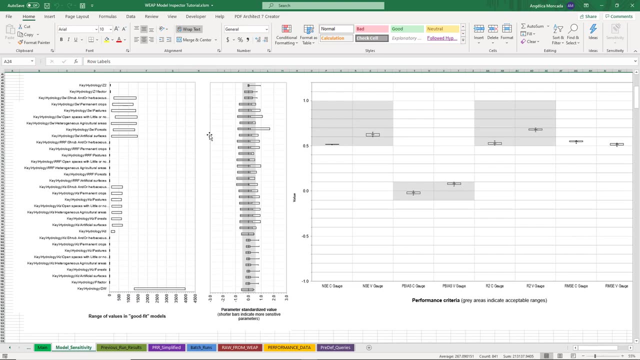 You can change the performance criteria, varying these values. Next you will have to apply the filter and get the results. This graph shows the values of the sets of parameters that meet the performance criteria. The first graph shows the interval of the parameters. The second one shows the minimum and maximum standardized values, with the mean. 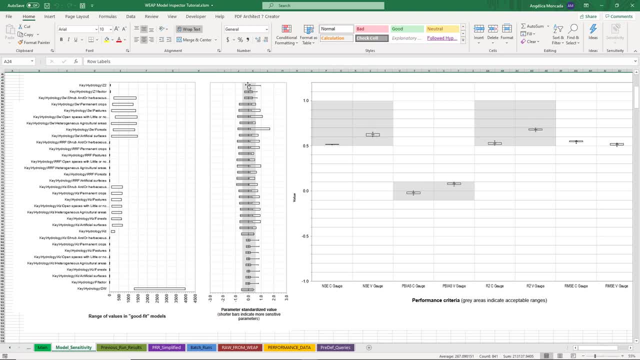 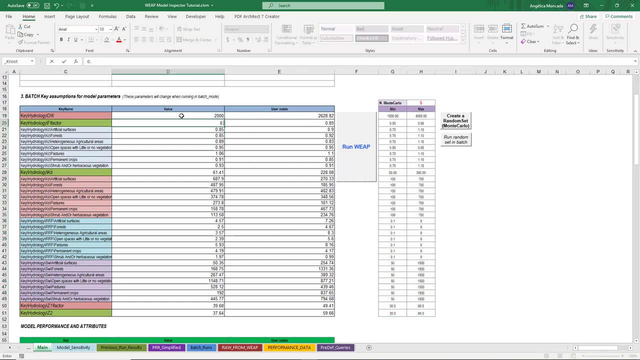 Shorter bars will show the most sensitive parameters. The third one is a box plot of the goodness of fit metrics. As you can see, the tool is useful to calibrate and validate the model systematically. You can vary the hydrological parameters and evaluate the performance of the model. You can continue exploring the tool. 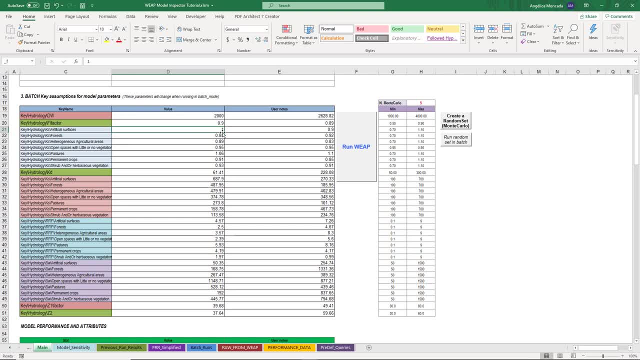 aiming to improve the performance of this model. The model is calibrated and validated when you find a parameter set that represents the water balance in the study area. the simulated streamflow represents the observed streamflow and the goodness of fit metrics meet the performance criteria. 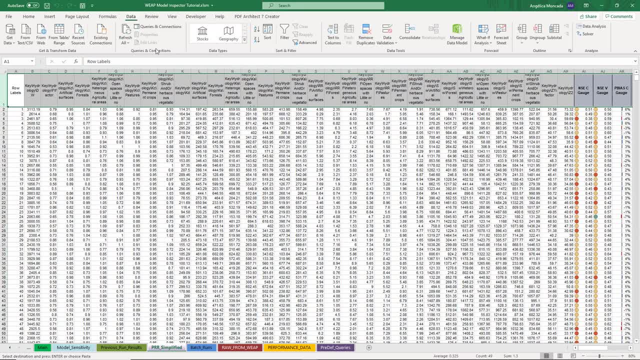 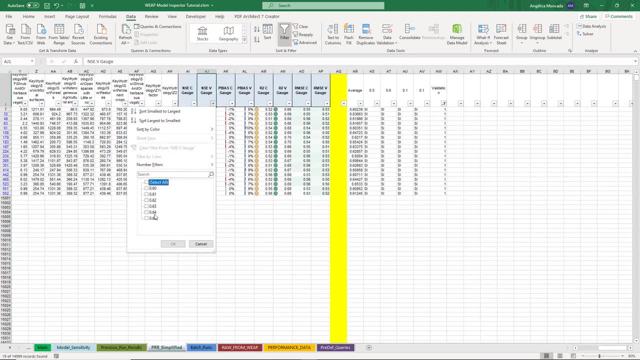 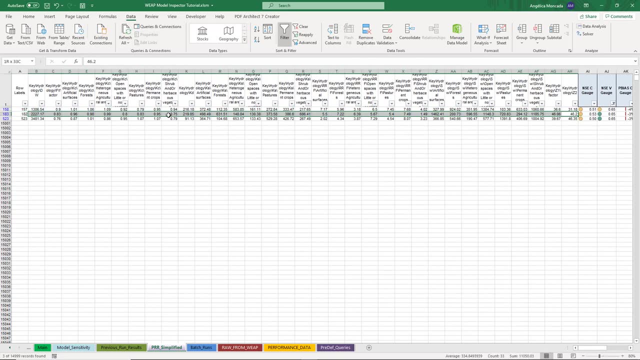 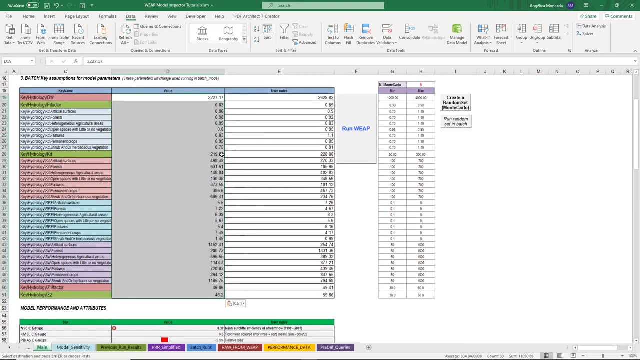 You can rerun the tool using the best set of parameters found so far. We could use the PRR simplified sheet. This is the generated table Filter: the parameter sets that meet the performance criteria. Copy and paste the values and run the tool again.